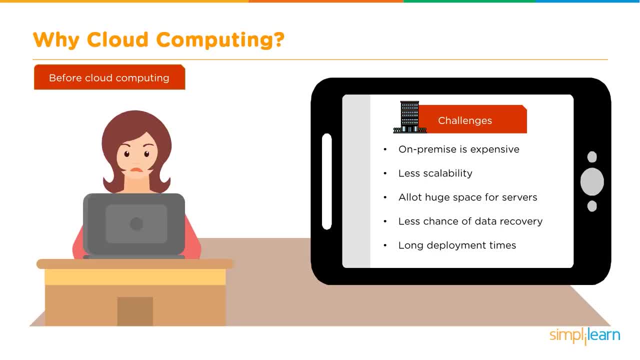 It is less scalable because you have already procured the infrastructure, So the scalability becomes lower. Along with that, they require a lot of huge space for the servers. If, in case, you have lost data in the on-prem, it becomes difficult to recover them. Along with that, it takes long deployment times. Apart from that, the 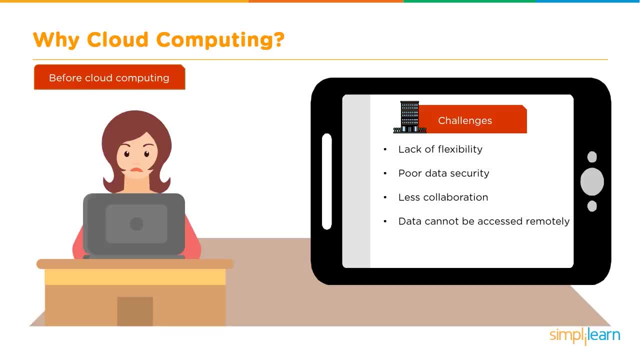 other challenges were the lack of flexibility, poor data security, less collaboration with the inter-infrastructure and the data cannot be accessed remotely- Though data can be accessed remotely, but there were some challenges in terms of the security. Now, all these challenges were basically over-exploited. 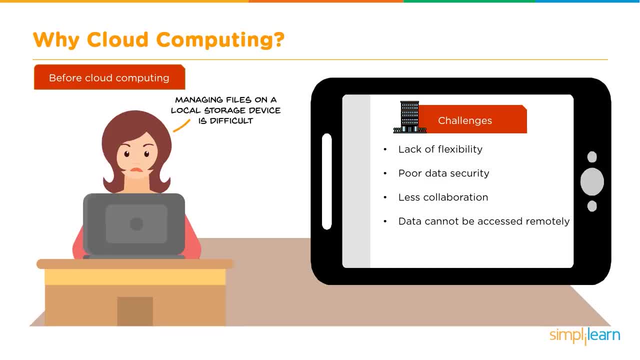 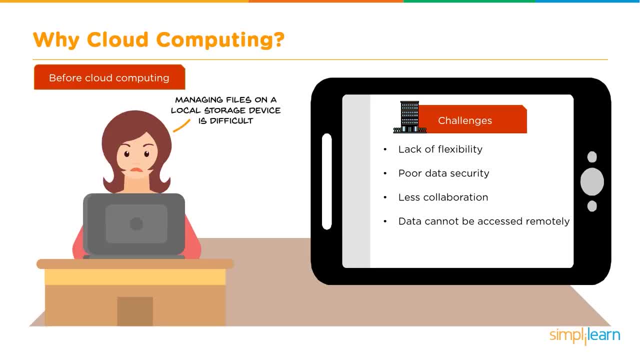 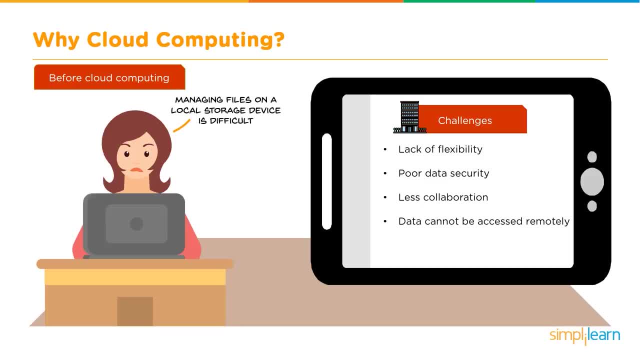 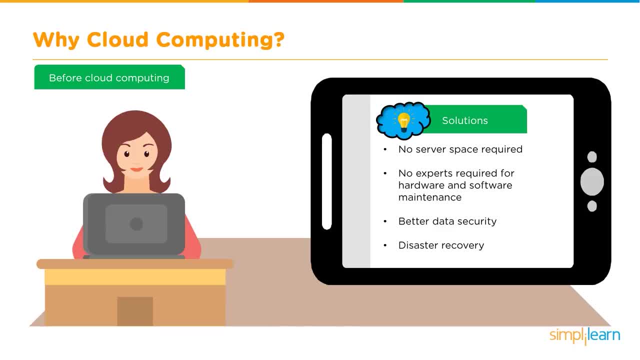 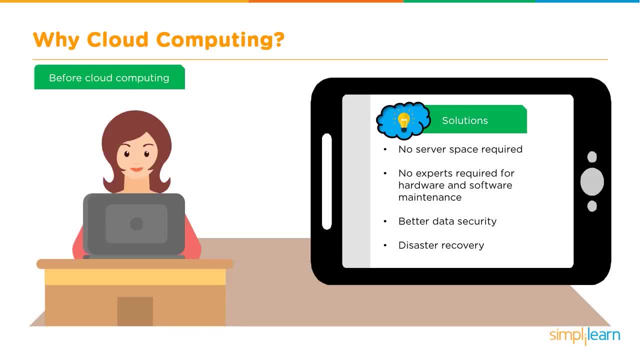 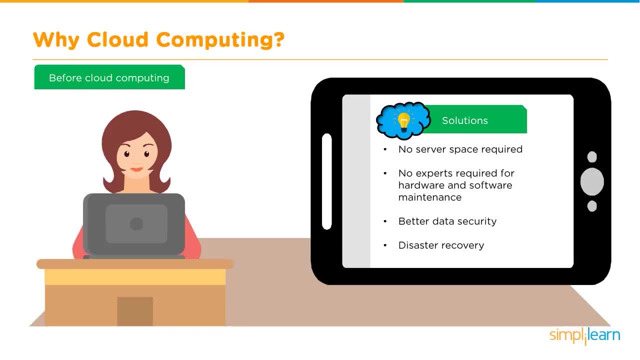 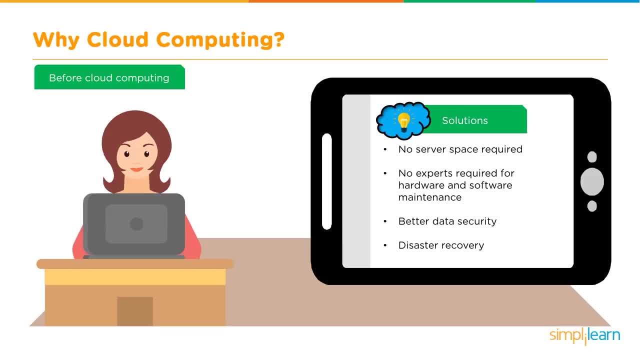 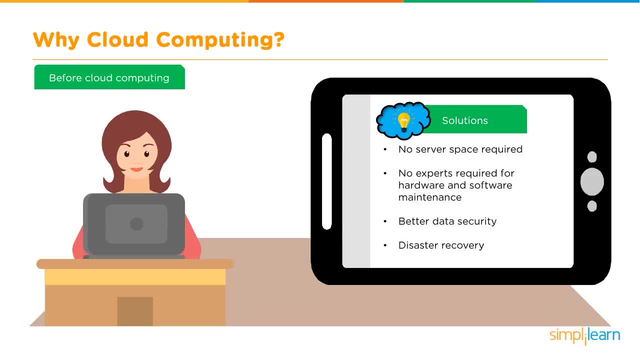 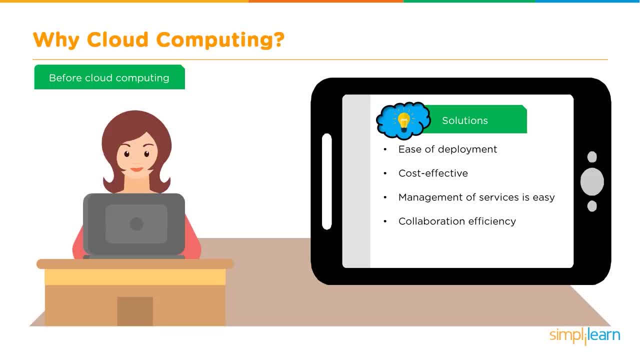 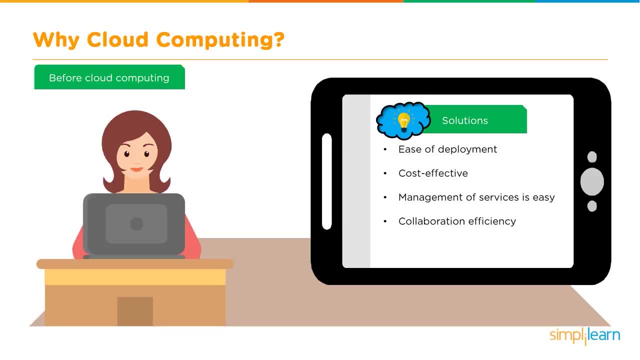 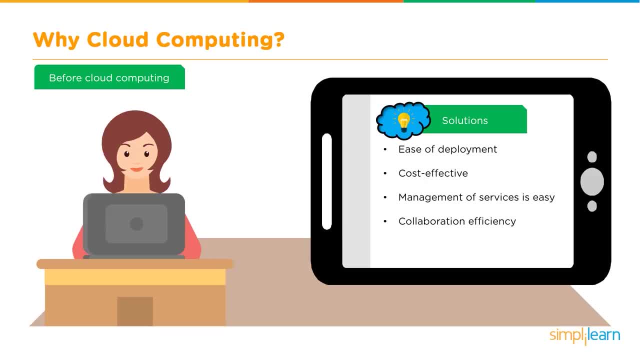 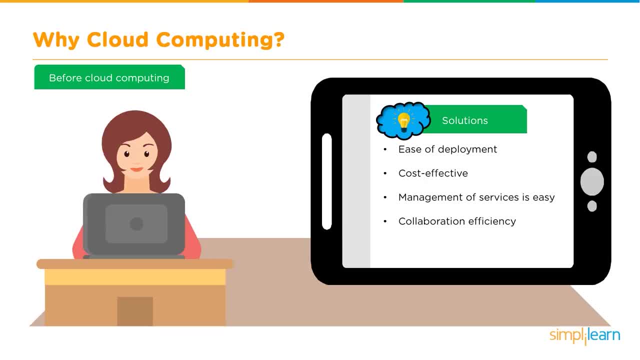 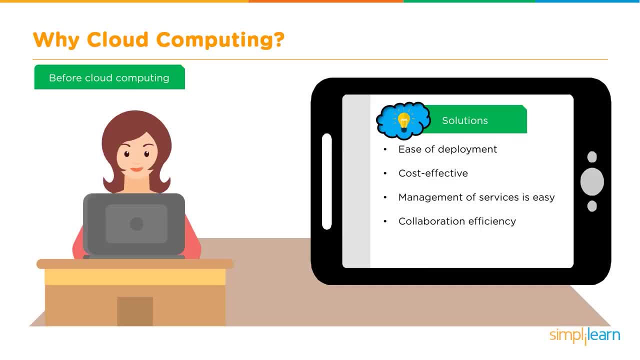 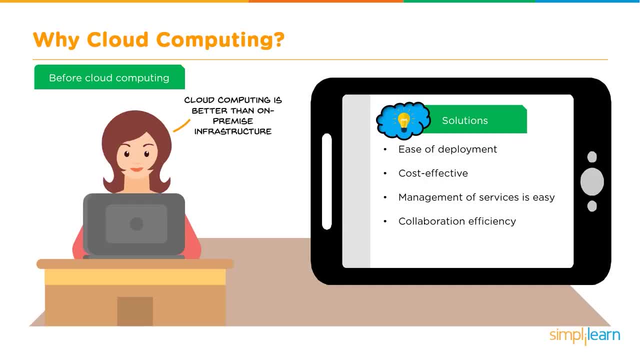 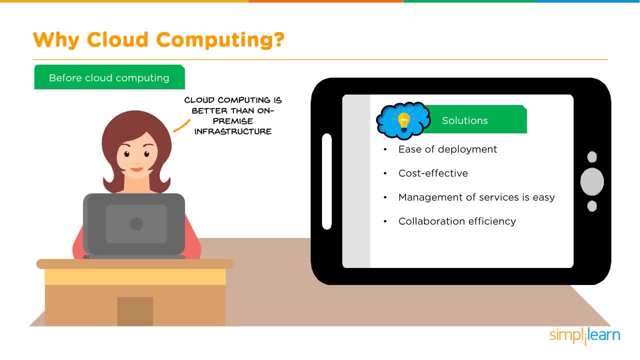 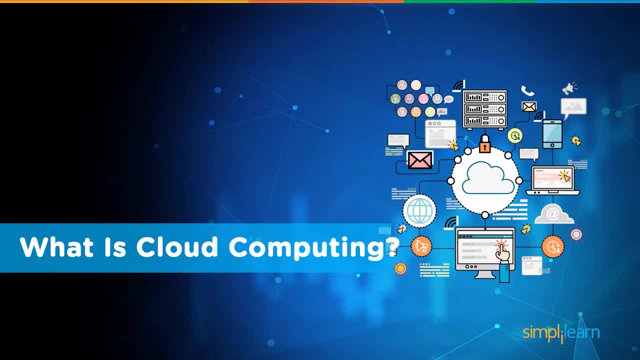 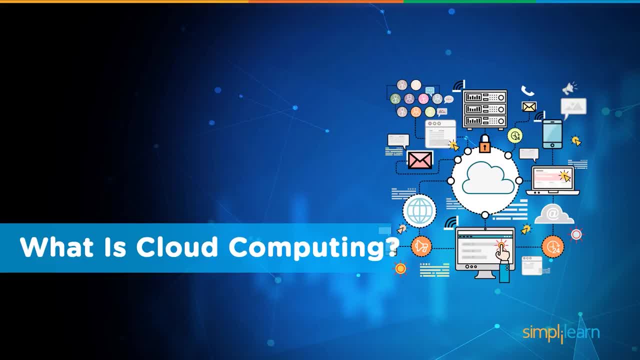 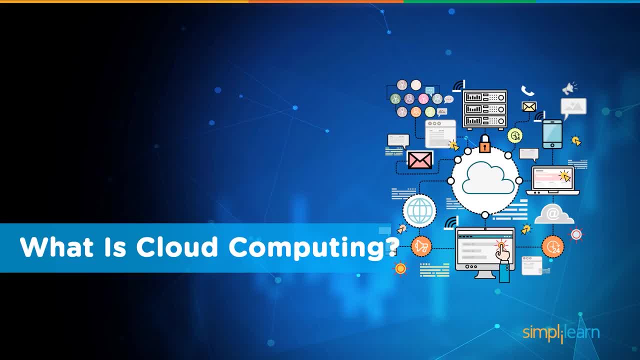 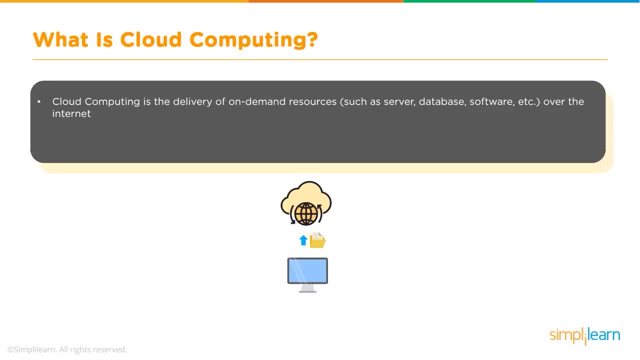 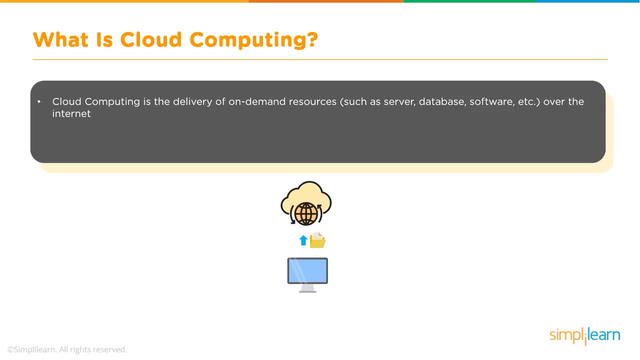 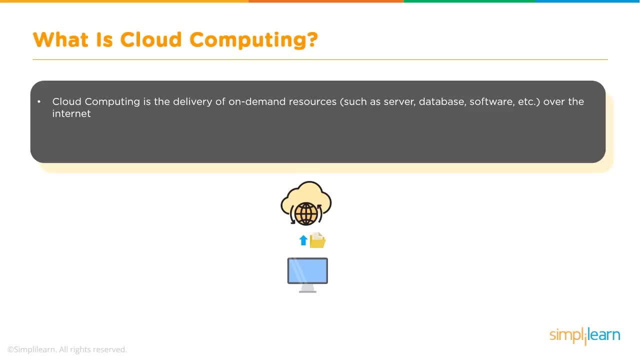 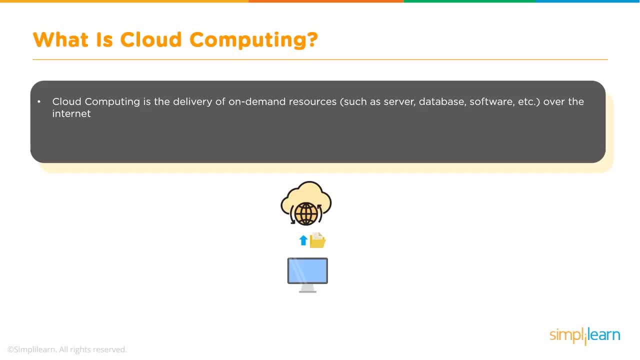 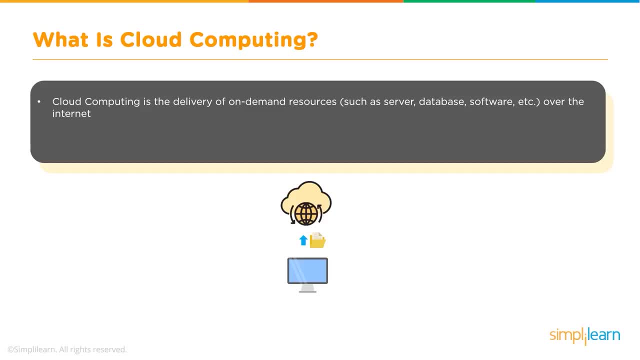 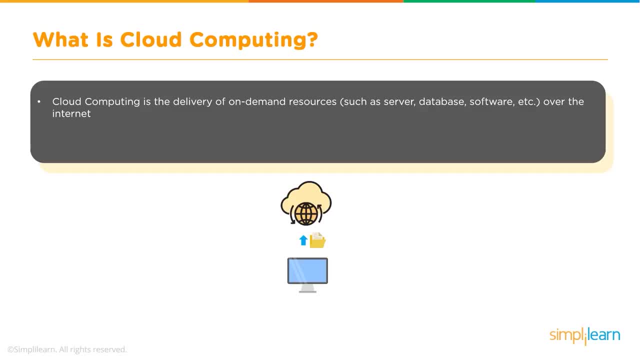 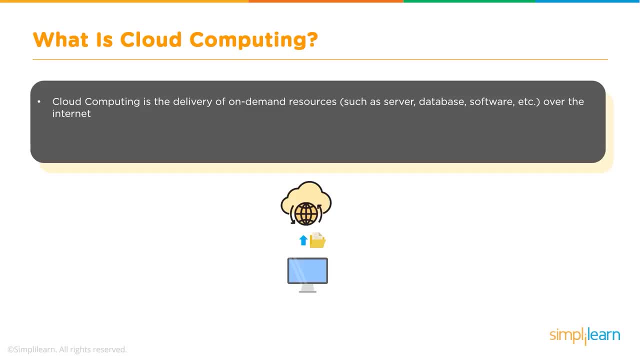 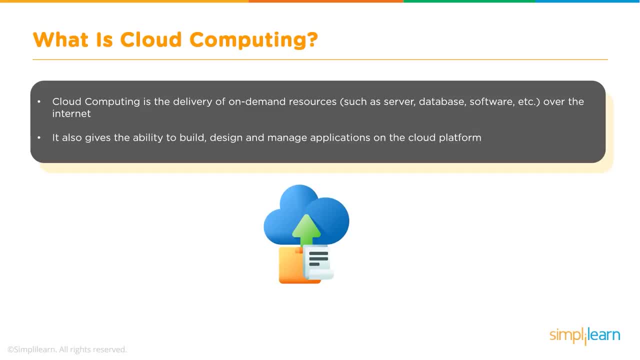 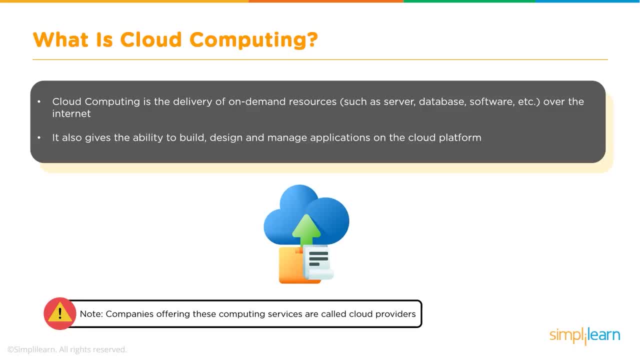 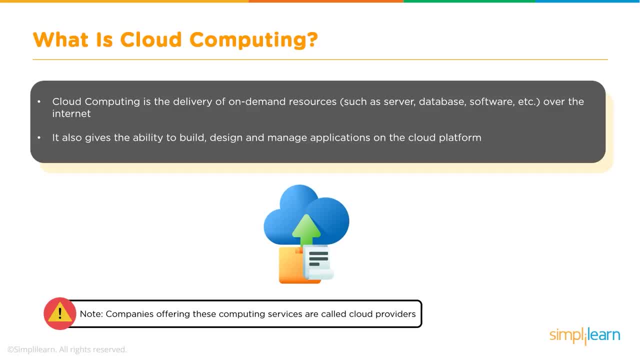 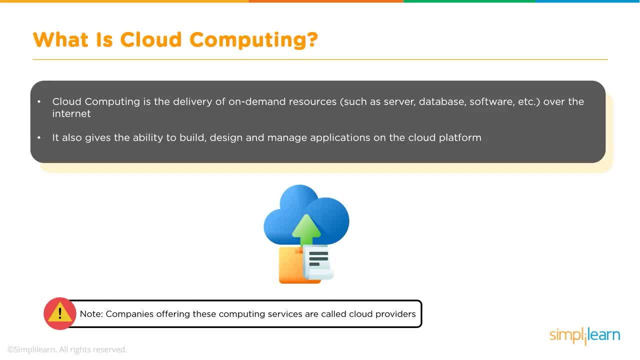 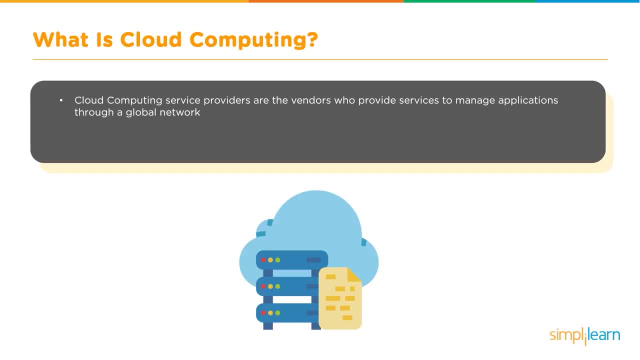 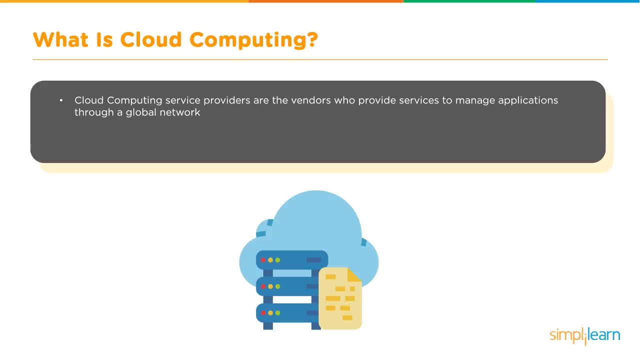 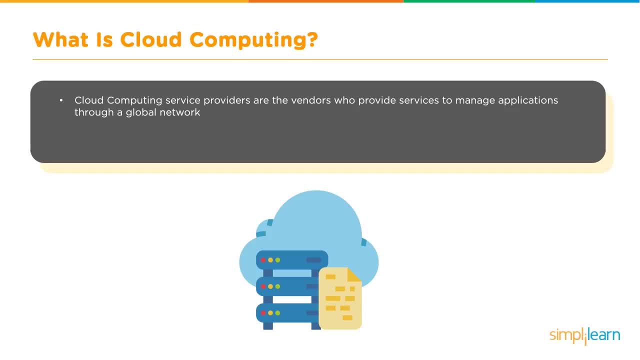 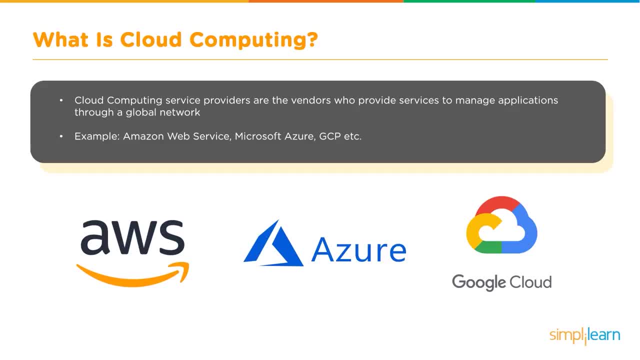 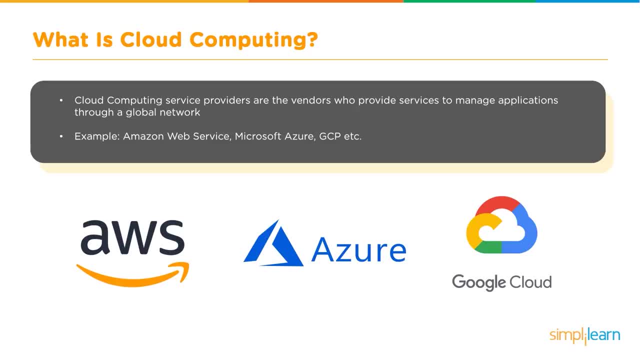 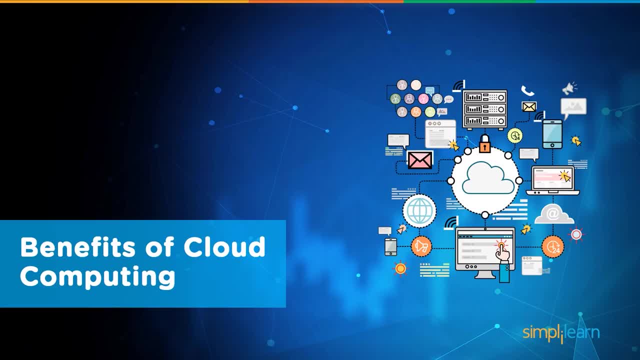 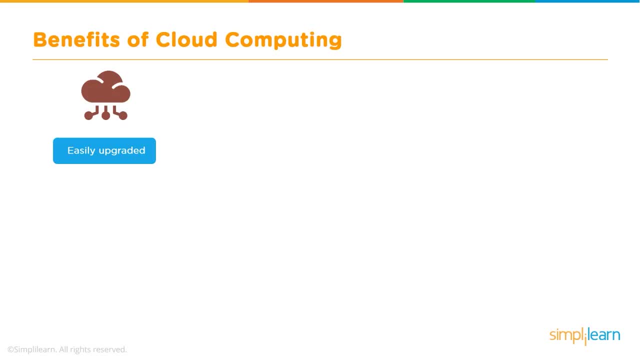 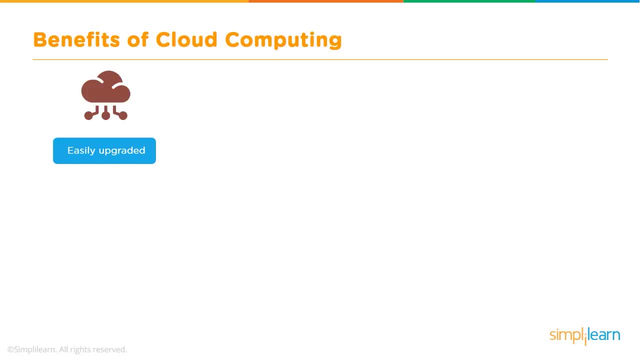 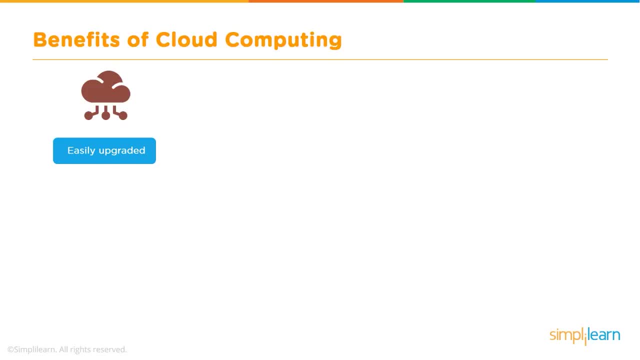 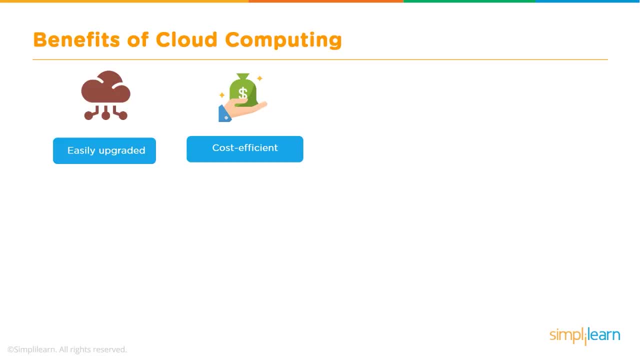 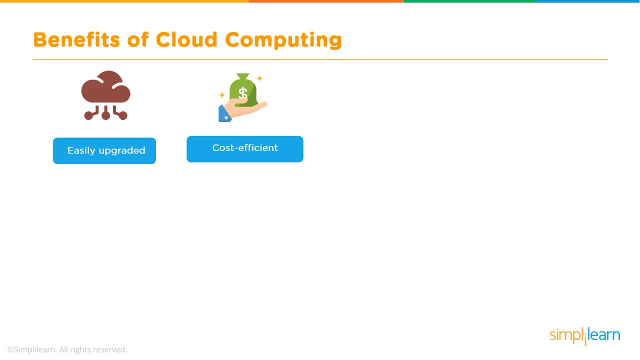 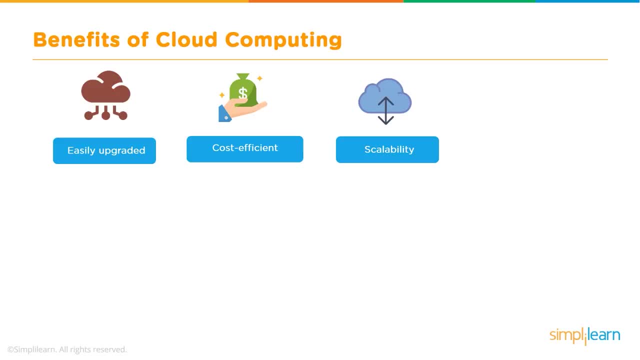 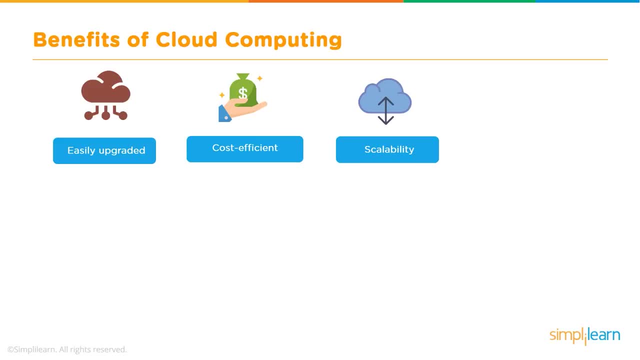 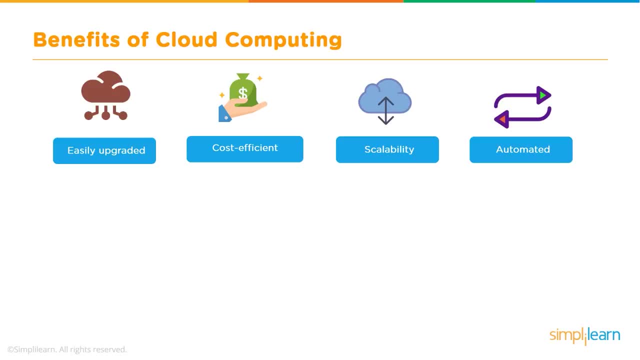 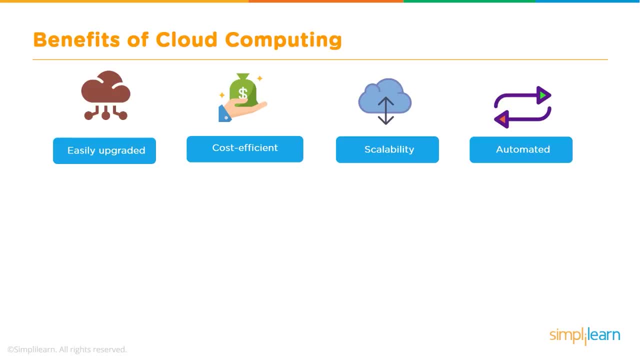 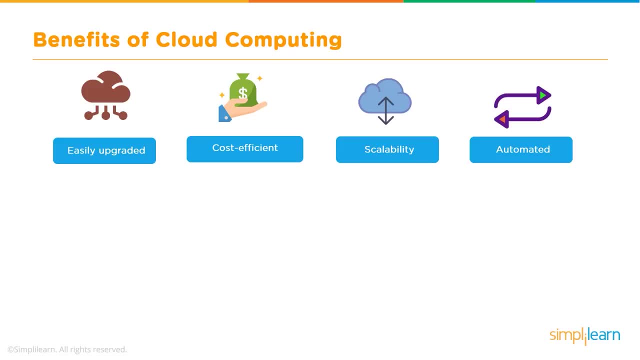 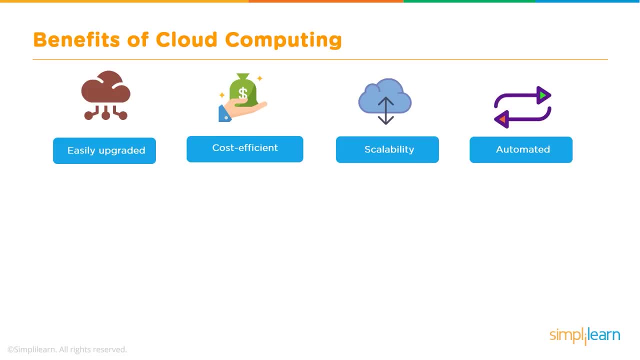 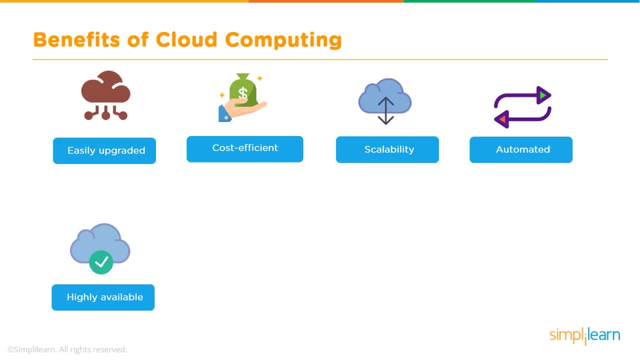 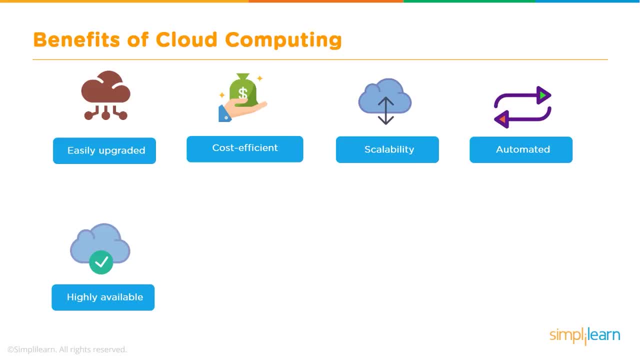 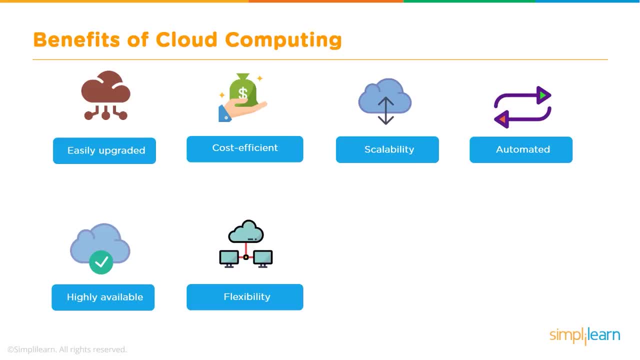 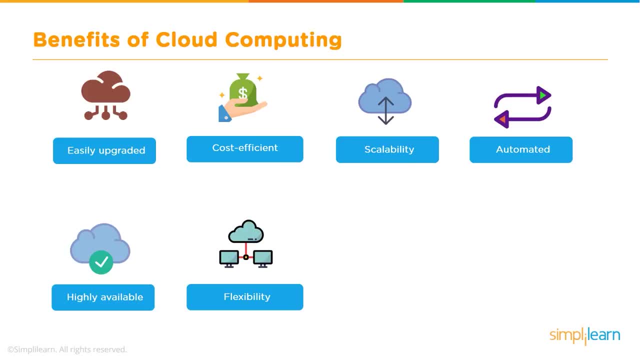 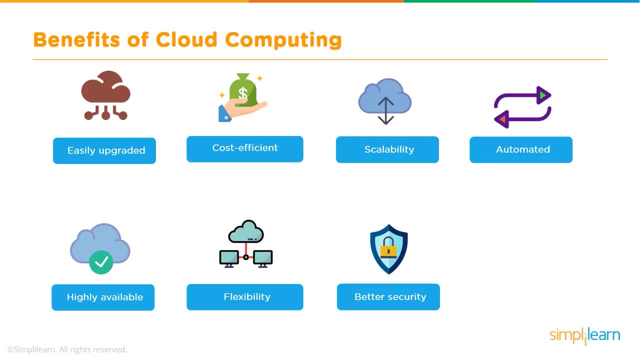 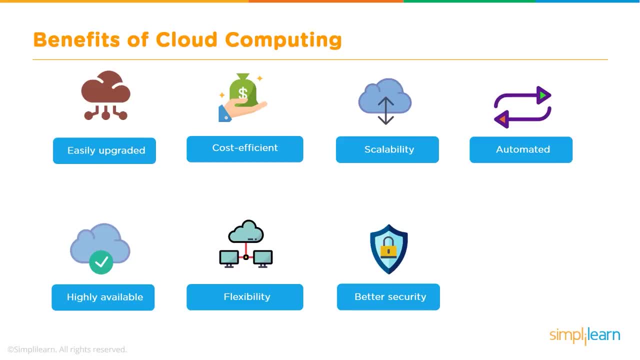 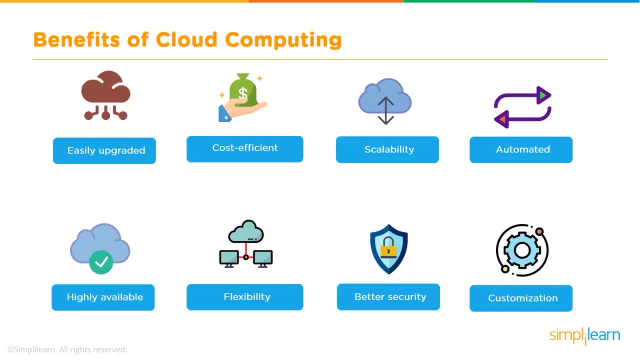 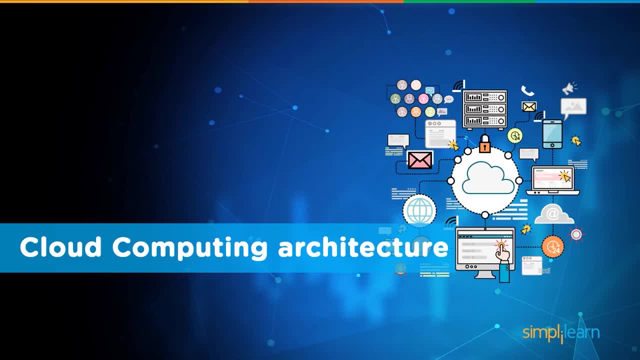 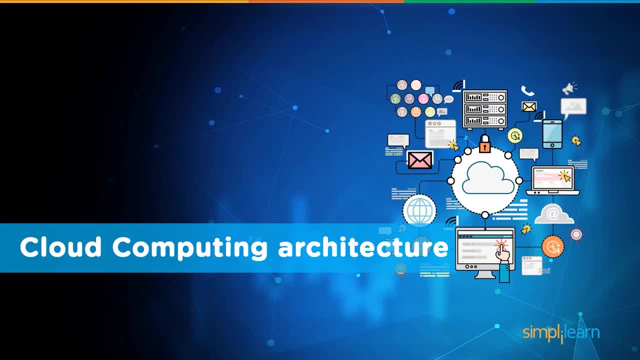 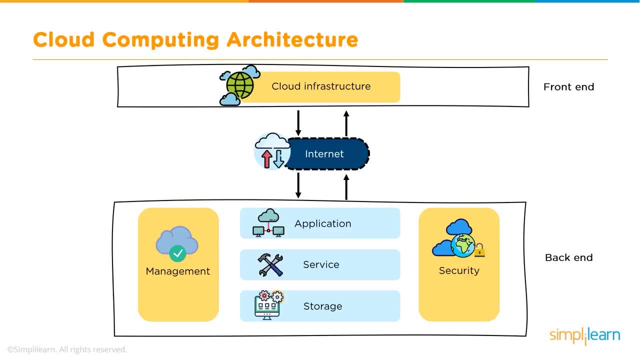 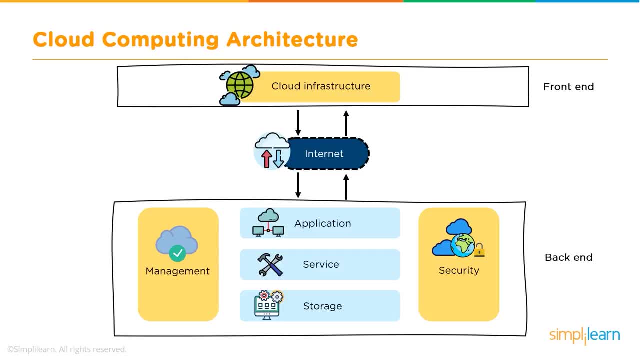 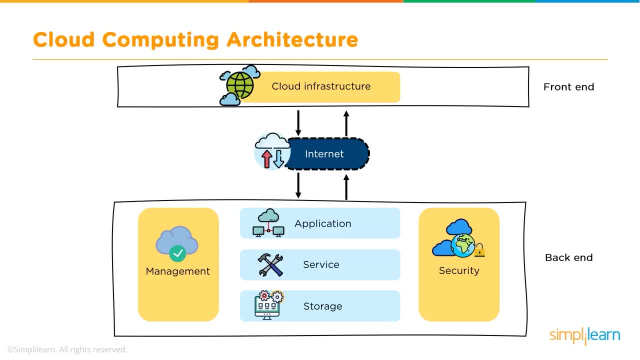 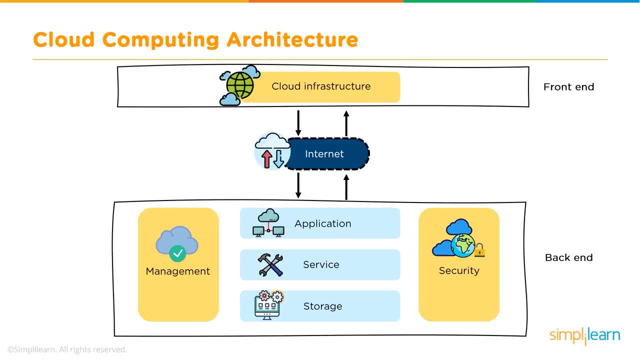 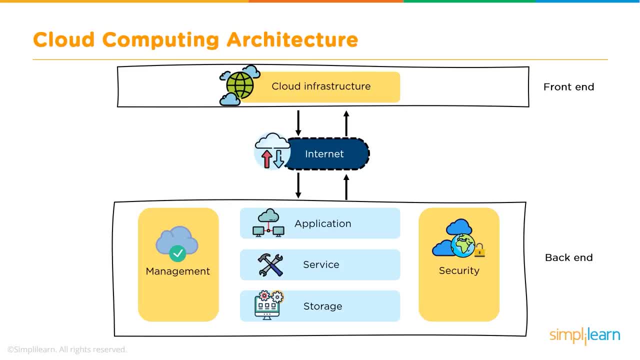 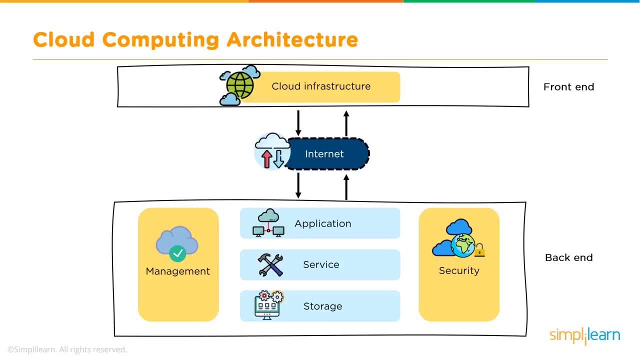 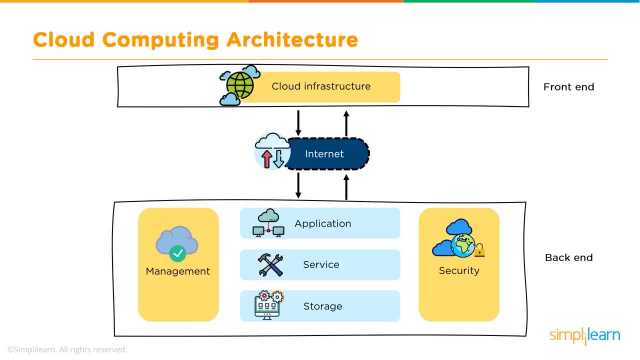 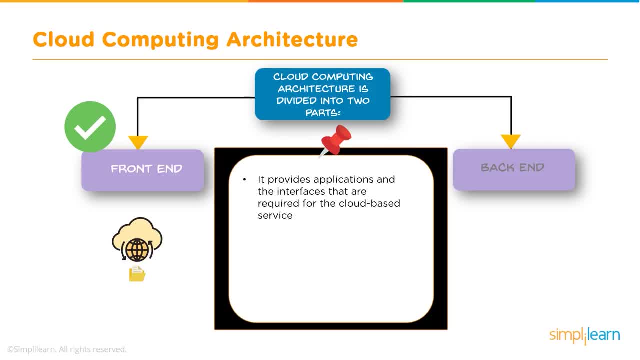 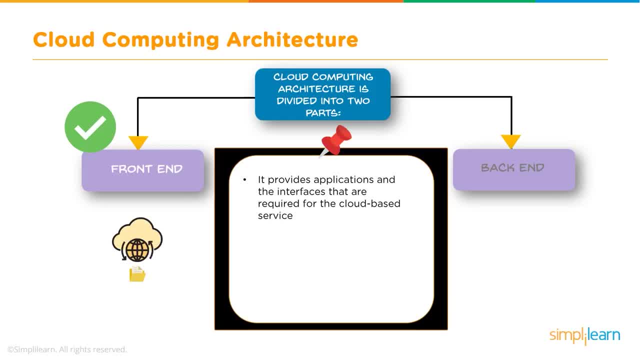 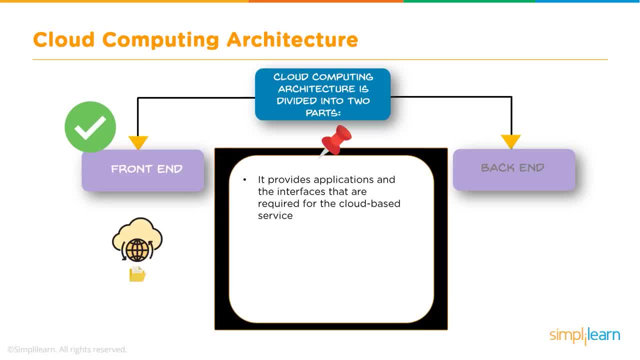 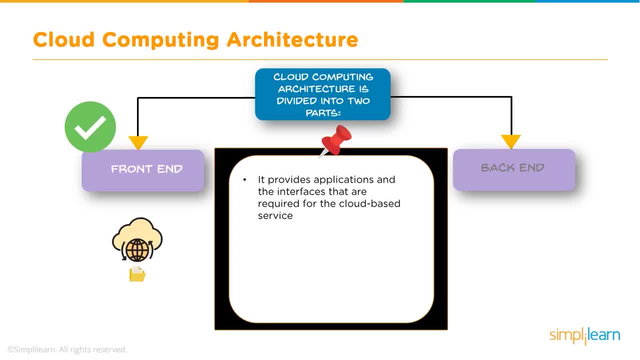 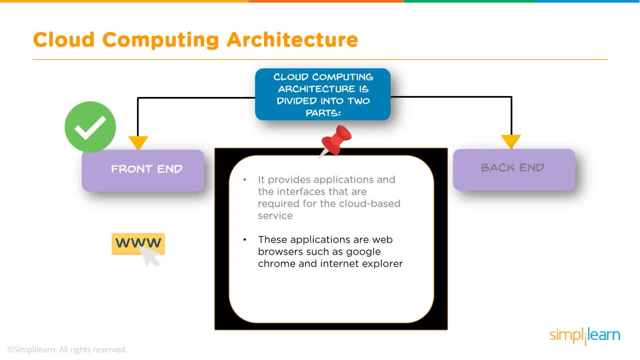 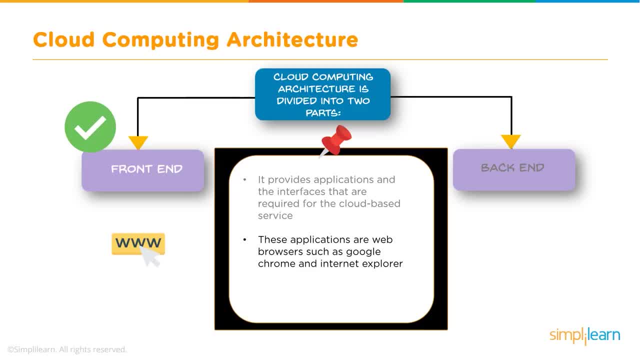 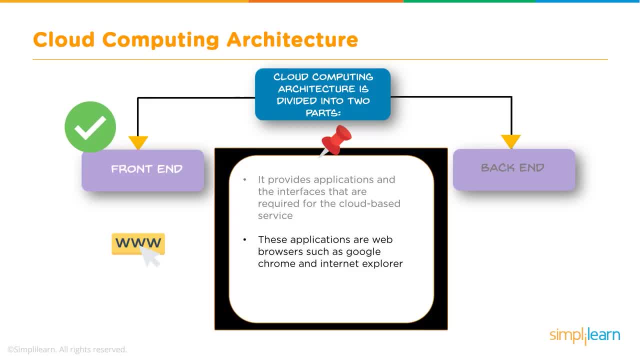 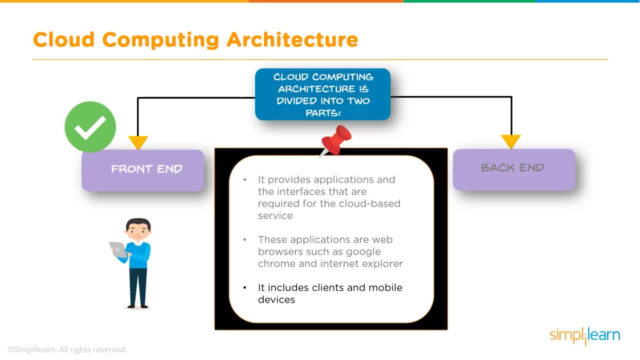 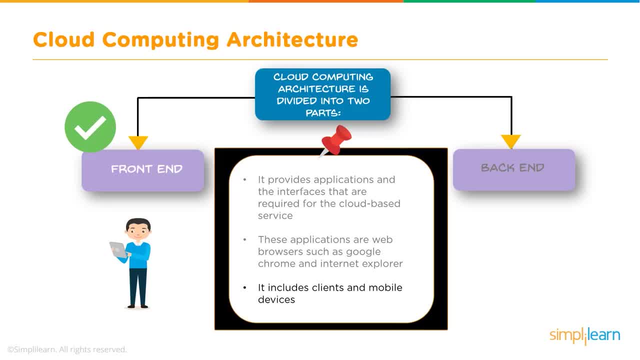 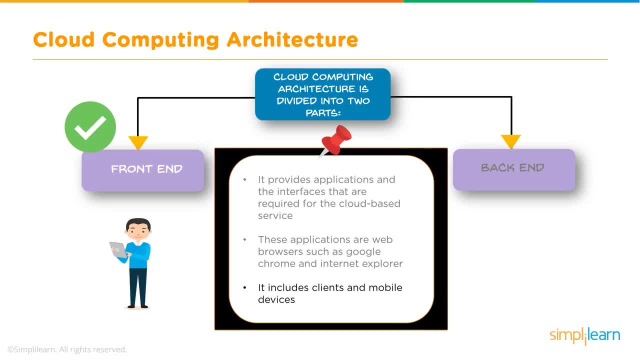 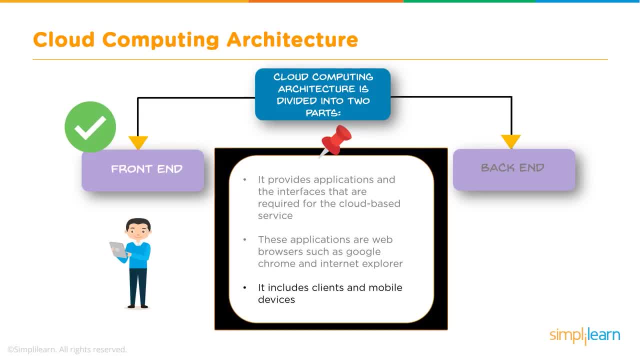 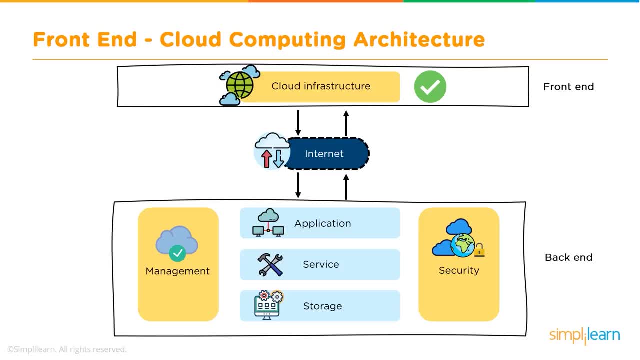 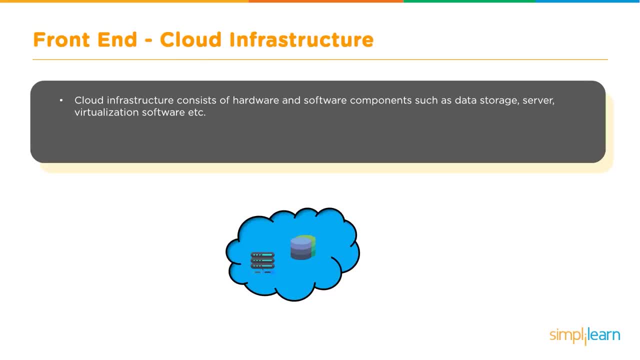 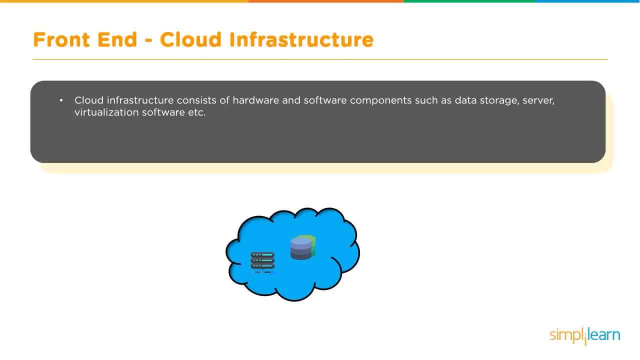 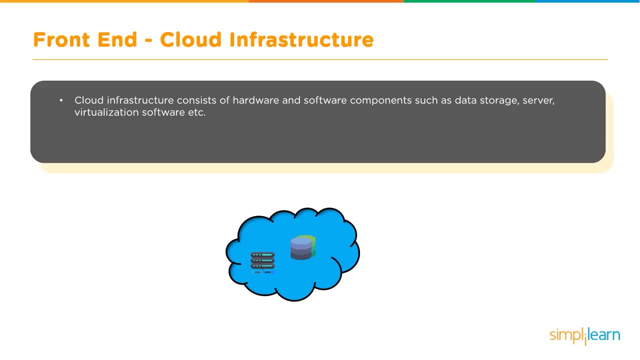 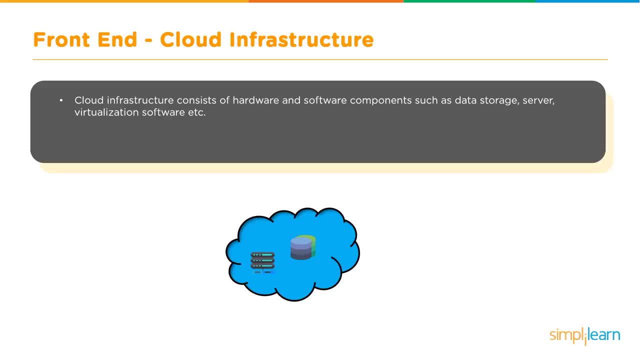 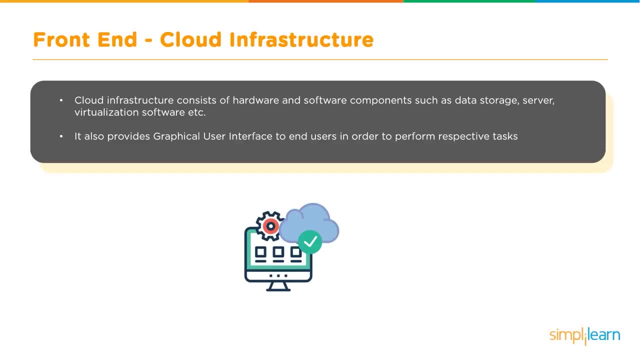 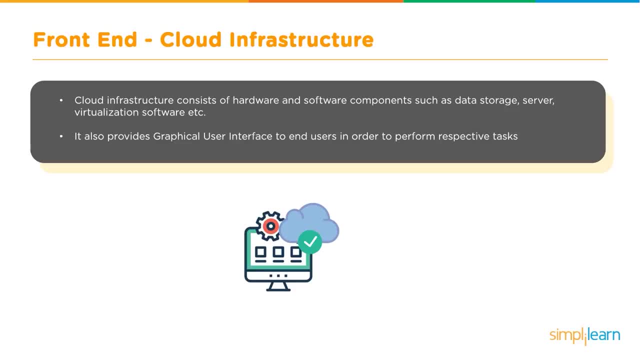 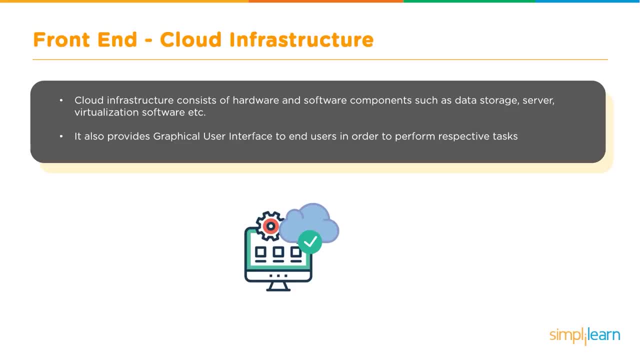 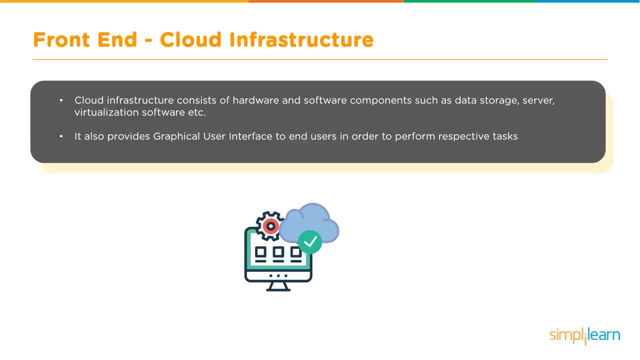 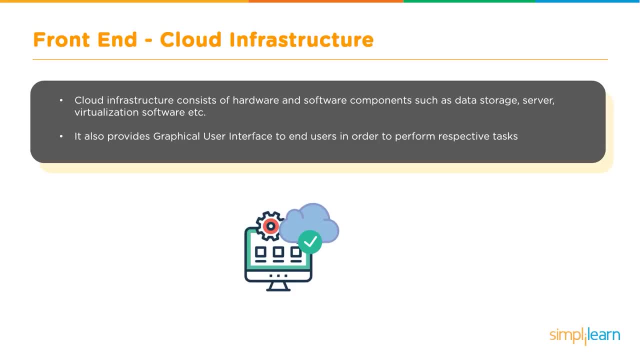 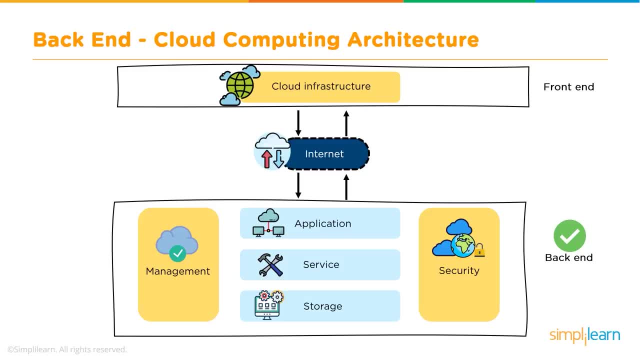 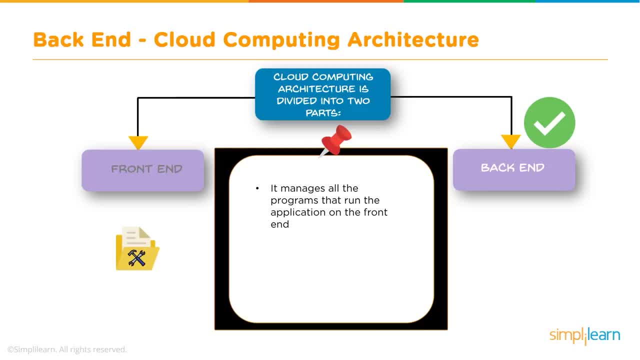 the programs that runs the application on the front end. so whatever is required to support the applications, for example web applications which are running on a front end, would be available in the backend. it has the larger number of data storage systems and server. so it is basically it. 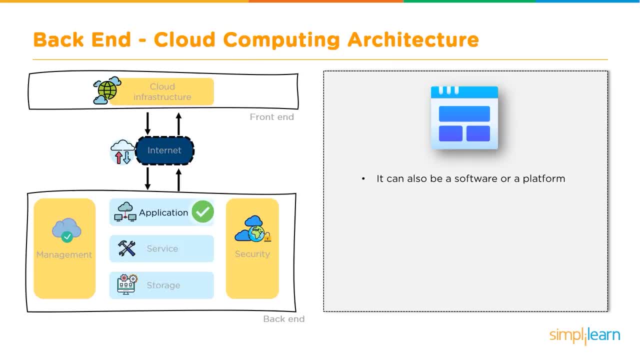 comprises of the entire infrastructure of a cloud provider, and it can also be a software or it can be a platform as well. so, based on the requirement, the application provides output to the end-users in the backend. also, it is one of the most important components in the cloud because it is, you can say, a 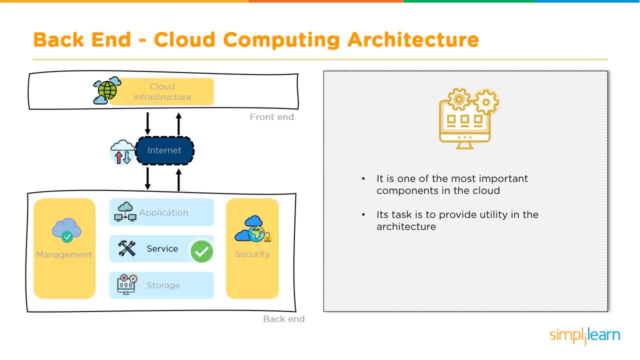 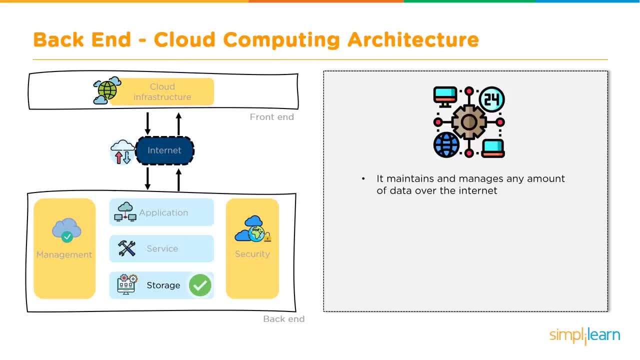 development environments and the web services in the backend, with respect to the storage it maintains and manages any time of any amount of data over the internet. some of the examples of storage services on the cloud are S3, which is called as a simple storage service, oracle, cloud storage and Microsoft. 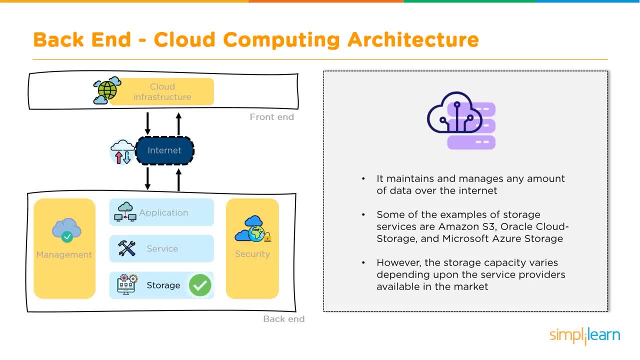 Azure storage. the storage capacity varies depending upon the service providers available in the market and also it allocates specific resources to a specific task. it handles functions of cloud environment. so this is with respect to the management in the back end architecture. the management in the back end architecture helps in the 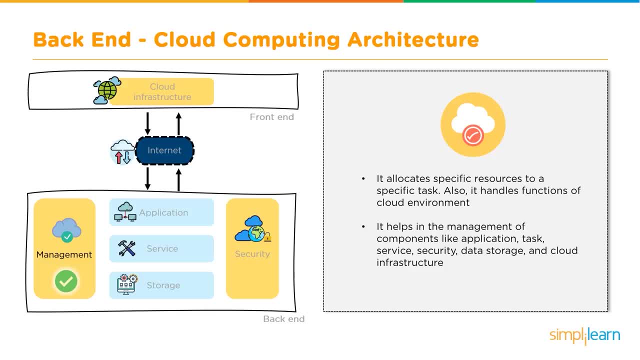 management of components like applications, tasks, service security, data storage and the cloud infrastructure and, in simple terms, it establishes coordination among the resources. coming to the security aspect of a back-end architecture, it is an integral part of a crowd infrastructure because, since you, it mostly relies on the storage and the databases, so it has to be more secure it. 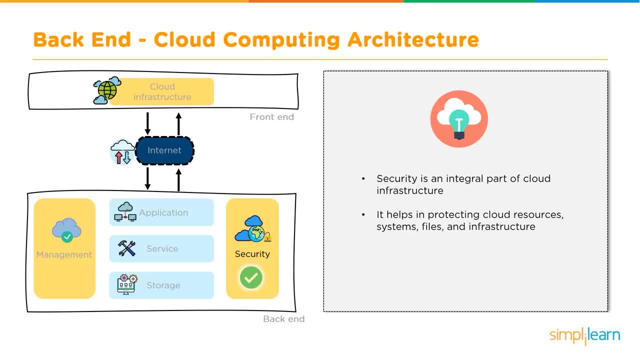 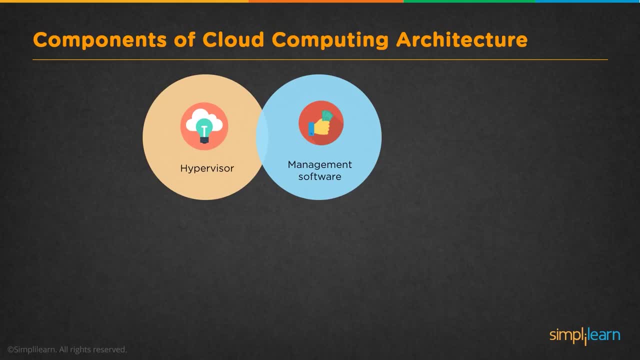 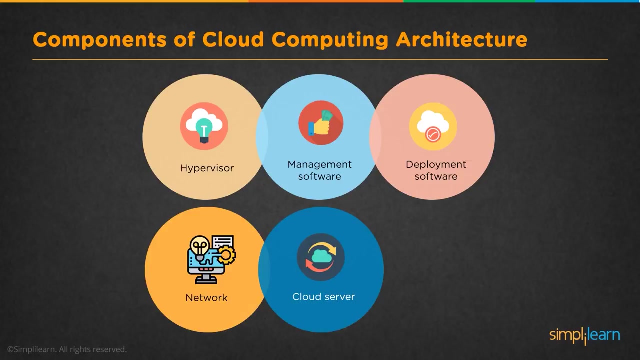 helps in protecting cloud resources, system files and the infrastructures. also, it provides security to the cloud servers with virtual firewalls and results in the prevention data loss. now the different components of the cloud computing architecture: one is the hypervisor. second is the management software. the third one is the deployment software. fourth one is the network. fifth, 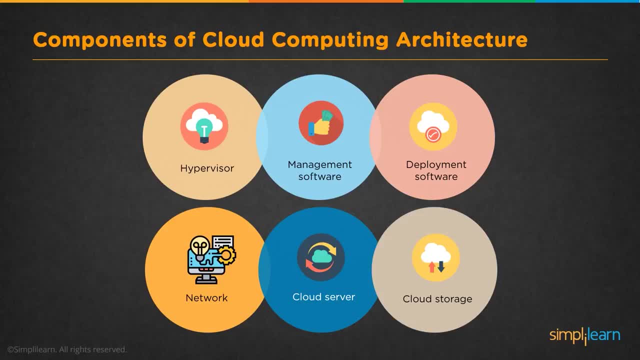 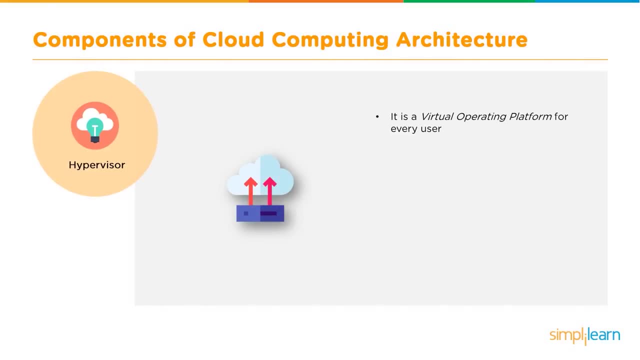 one is the cloud server and you have the cloud storage. now let's look into what we have with the hypervisor. hypervisor, as the name suggests, it's a virtual operating platform and that is basically used by every user. it runs a separate virtual machine on the back-end. 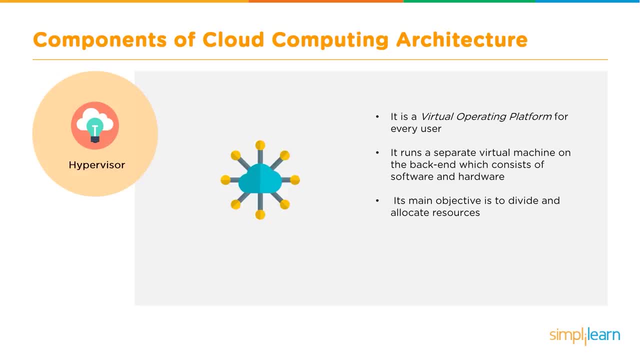 which consists of a software and the hardware. also it maintain objective. its main objective is to divide and allocate resources. so basically, the hypervisor is primarily used to virtualize the physical machines so that it can be shared across with many resources or many users. the management software- its responsibility- is to manage and monitor the cloud operations. so all 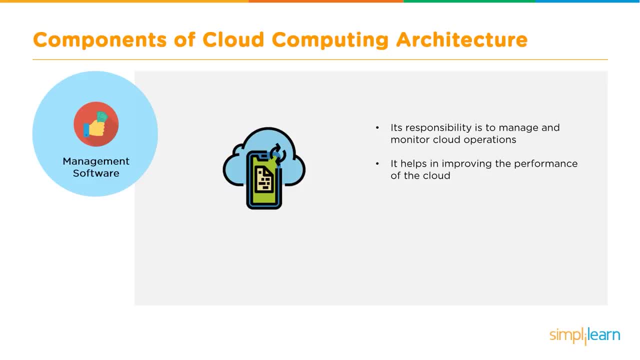 the operational tasks are basically done by the management software. it helps in improving the performance of the cloud, since you can do the admin task as well. for example, high security, flexibility, full-time access and the access given to other users who would be working on the cloud platform. the deployment software consists of all the mandatory installations and configurations. 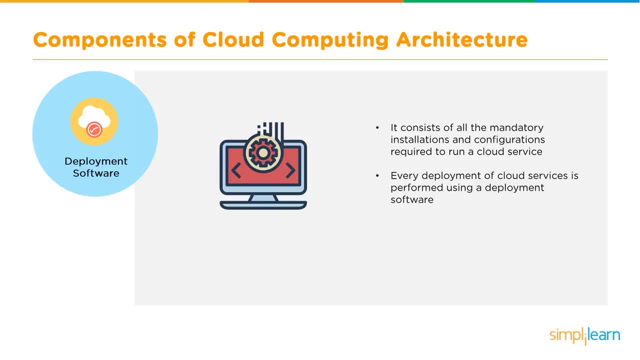 that are required to run a cloud service. every deployment of cloud service is performed using a deployment software, so it is primarily used for deploying the applications or a software, so that basically saves the time of a developer in terms of deploying their codes. now the three different models which can be deployed are the software as a service, which we call as a sas, so the software. 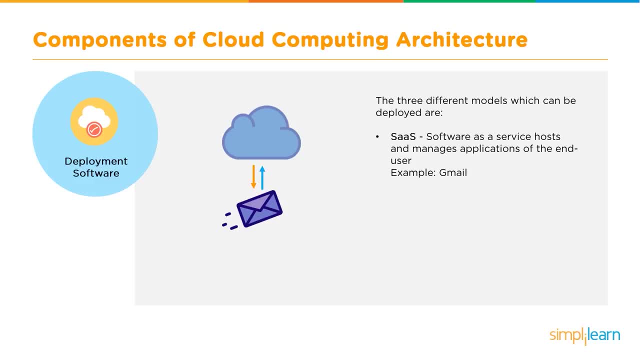 as a service means it hosts the software and manage the application of the end user. example is gmail. so gmail is an example of a sas service where it acts as a mailing service and the users just have to create their email accounts and start using the service. 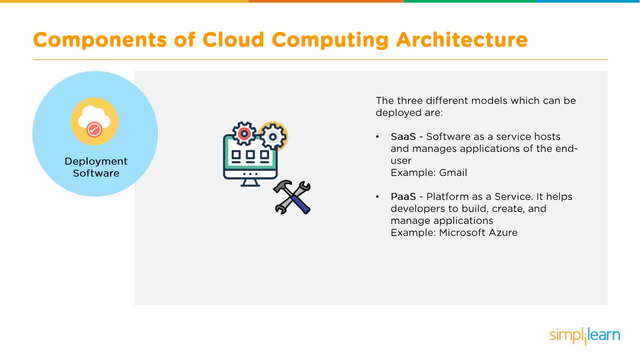 the pass is basically a platform as a service and it helps to develop and build and deploy the applications and the software primarily used by the coders. they can concentrate more on their development activities and less focus on the infrastructure. part example is microsoft azure and the infrastructure as a service. ias is basically to provide services on pay as you. 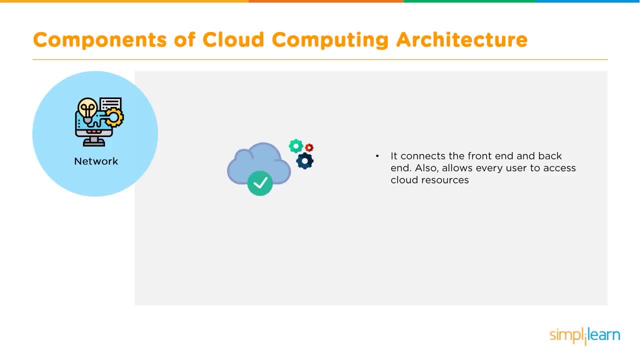 go pricing model. uh, coming to the component of a cloud computing architecture, that is, network. so what is with respect to network? why do we need a network? so it connects the front end and the back end together. so the network can be the internal private network of a cloud computing provider, as well as the 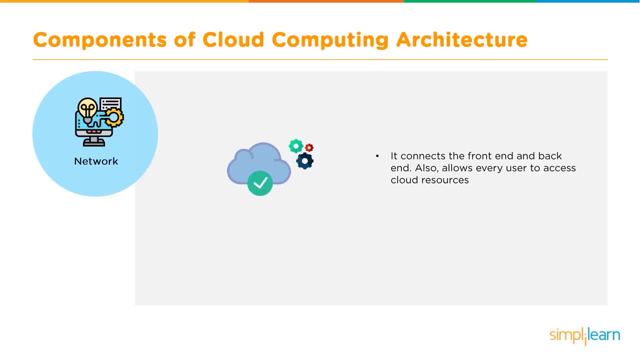 public network and also it allows every user to access the cloud resources over the internet. it helps users to connect and customize the route and protocol. so let's say an admin wants a particular ips to be blocked, so you can specify them and customize them in the route and the protocols. it is a virtual server which is hosted on the cloud computing. 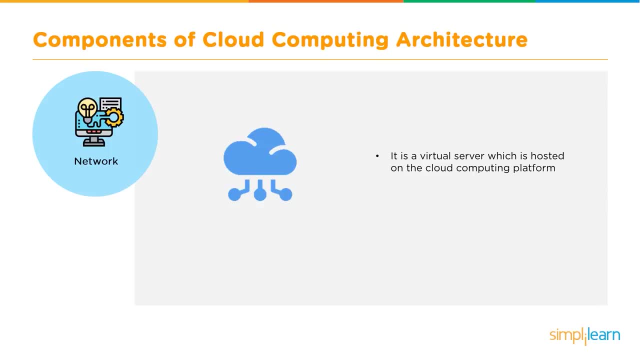 architecture, so it is just like a virtual networking that is available on the cloud computing platform. it is highly flexible, secure and cost effective and it is basically, you can say, the backbone in terms of connecting multiple services together. the cloud storage is basically where every data is stored and that can be accessed by a user from. 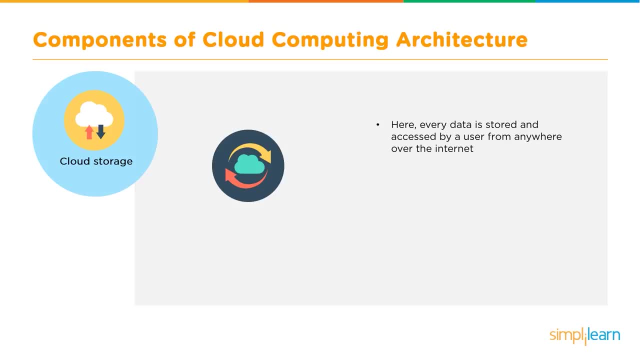 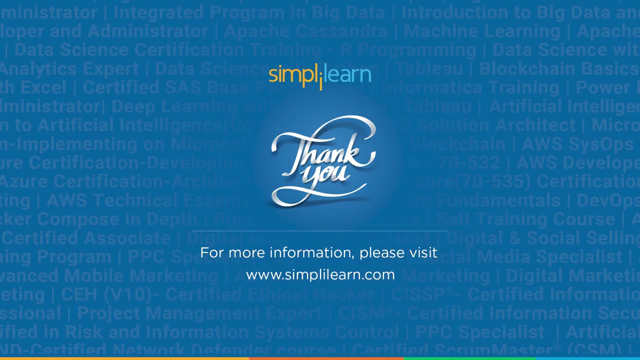 anywhere over the internet. of course, it depends on how do you provide the access to it. it is scalable at runtime and it is automatically accessed, and the data can be modified and retrieved from the cloud storage over the internet itself. so this was about our session for today. guys, thank you for watching this video. 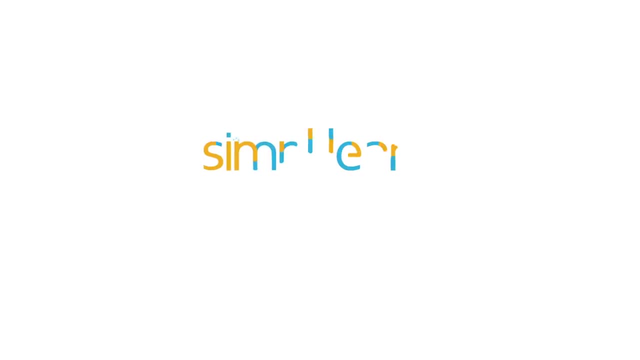 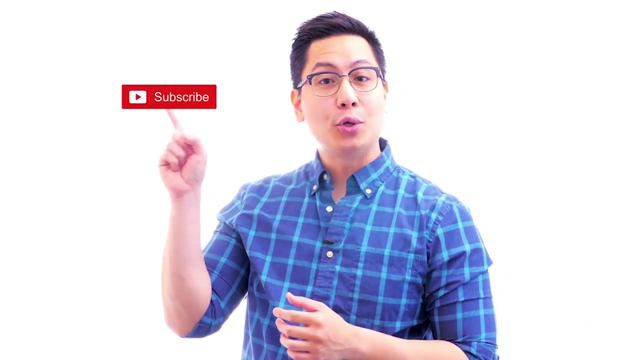 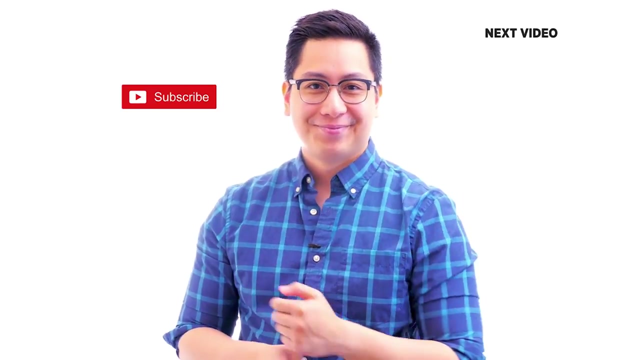 i hope you like it, hi there. if you like this video, subscribe to the simply learn youtube channel and click here to watch similar videos. to nerd up and get certified: click here.